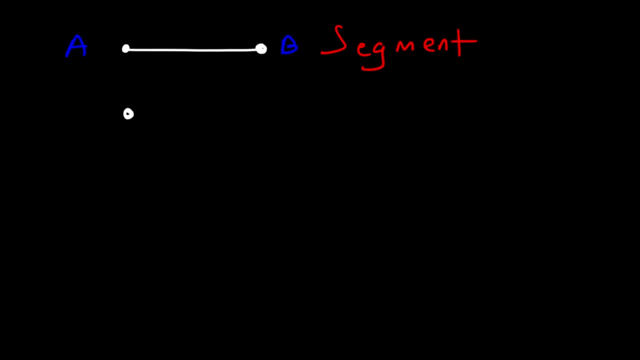 A ray has one endpoint and the other side goes on forever. So that's a ray. A line has no endpoints. A line extends forever in both directions. So when we're talking about angles, an angle is formed between two rays and it has a common endpoint, which is right here. 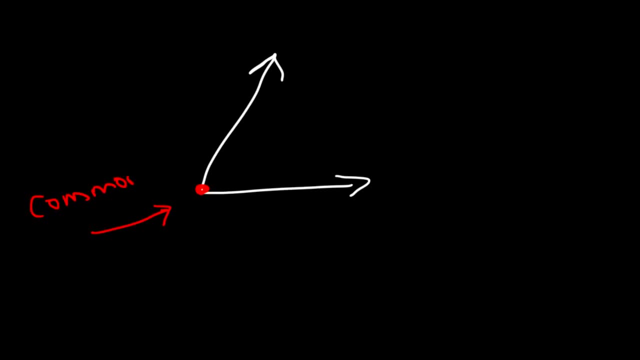 This endpoint is also known as the vertex of the angle. The first ray is known as the initial side, The second ray is known as the terminal side, And the angle, which we can call theta, is measured from the initial ray to the terminal ray. 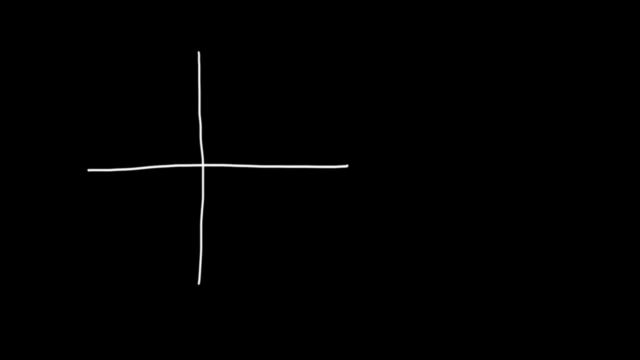 Now let's say, if we have a graph with the x-axis and the y-axis, An angle is said to be in its standard position if the vertex is at the origin, so that's the common endpoint, and the initial side, or the initial ray, is on the x-axis. 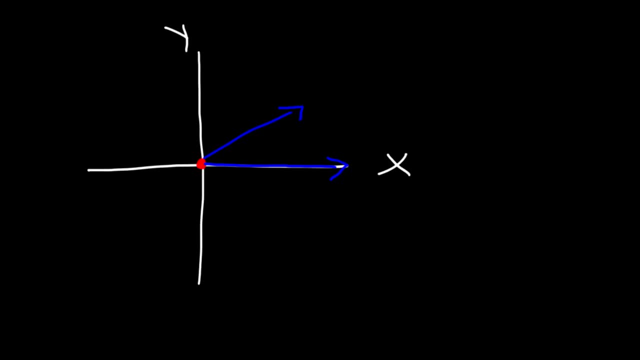 Now, if the terminal side or the terminal ray is above the x-axis, in this case, if we rotate the angle, or if we rotate from the initial side to the terminal side in the counter-clockwise direction, then the angle is going to be positive. 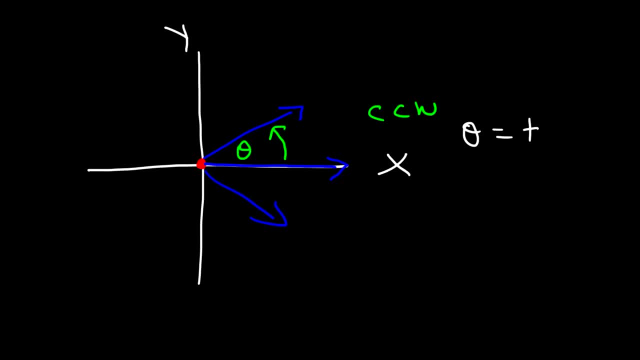 If we need to rotate towards the clockwise direction in order to go from the initial side to the terminal side, then the angle is negative. So, for example, let's say, if we want to draw an angle of 30 degrees, This would be an angle of positive 30 degrees. 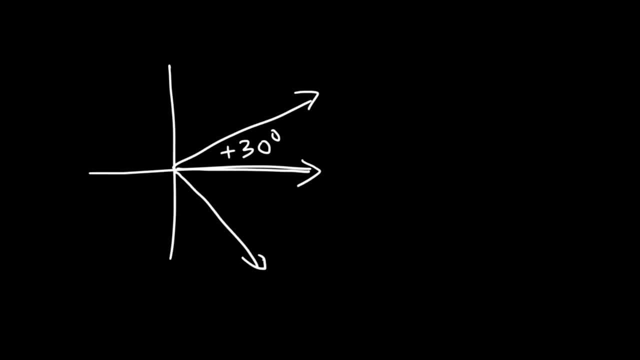 If we want to draw an angle of negative 45, we would have to travel in the clockwise direction, so this would be an angle of negative 45 degrees. Now, what is the difference between an acute angle, a right angle, a straight angle and an obtuse angle? 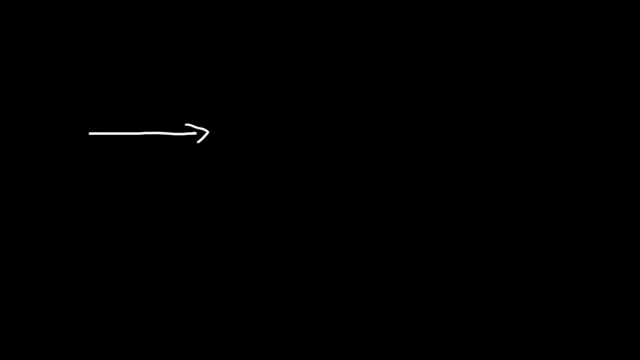 You need to know the differences between the four. So in geometry you've learned that a right angle is a 90 degree angle. Sometimes you'll see this box, So that's a right angle. The next angle that you need to be familiar with is an acute angle. 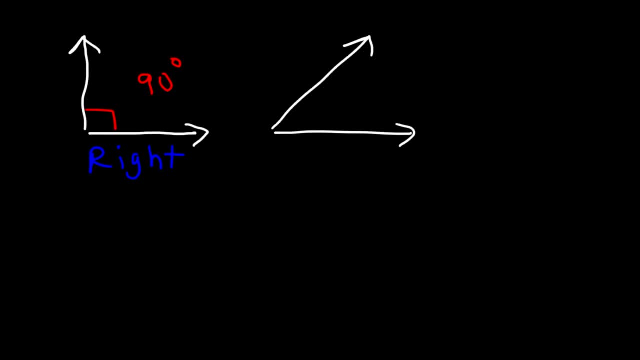 An acute angle is simply an angle that's less than 90 degrees, but that's greater than zero. So 60 is an acute angle. Now what about a straight angle? A straight angle is basically equivalent to a straight line. It has an angle of 180 degrees. 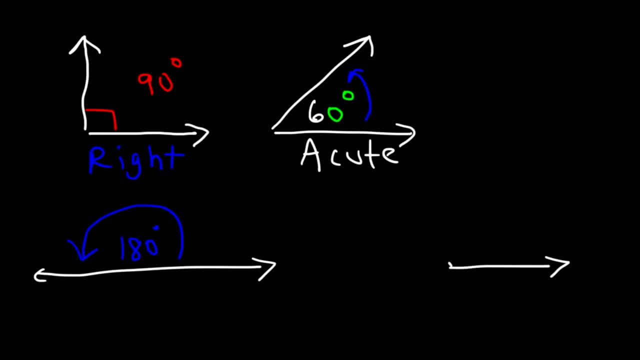 Finally, we need to go over an obtuse angle. So let's say this is the terminal side and here's the initial side. An obtuse angle is greater than 90. So in this case, let's say the angle is 130 degrees. 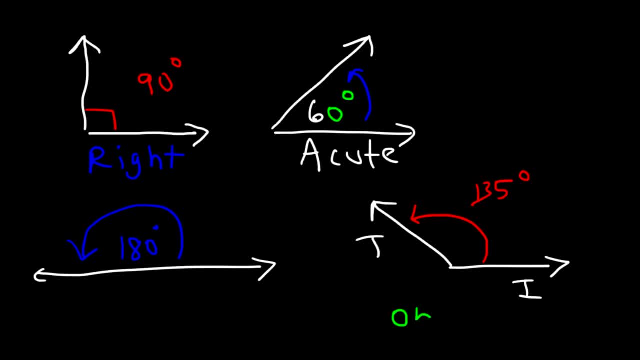 That means this one is an obtuse angle And this is called, as we mentioned before, a straight angle. So make sure you're familiar with these terms. Now you need to be familiar with the four quadrants. This is the first quadrant. 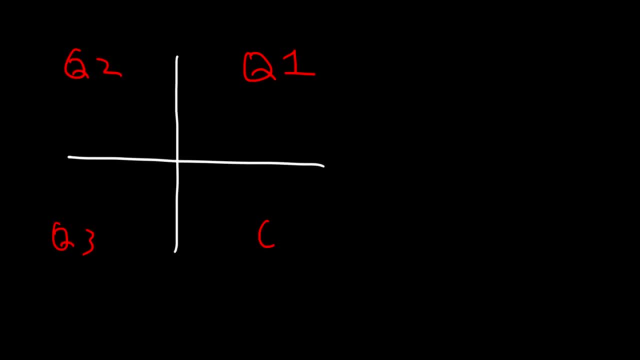 Here you have the second. This is the third quadrant And this is the fourth quadrant. X is positive in quadrant 0.. X is positive in quadrants 1 and 4.. Y is positive in quadrants 1 and 2.. 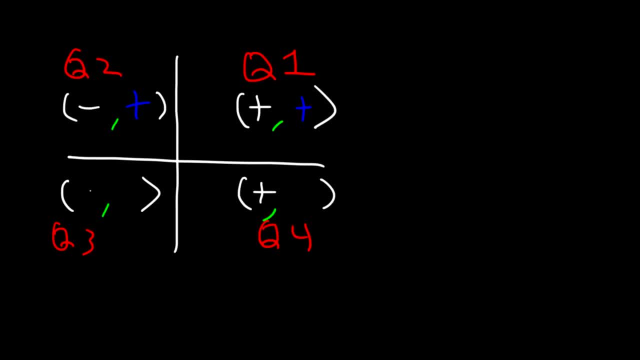 X is negative in quadrants 2 and 3.. And Y is negative in quadrants 3 and 4.. So make sure you know that, Particularly, as we get into sine and cosine, Because sine is associated with the Y values, Cosine is associated with the X values. 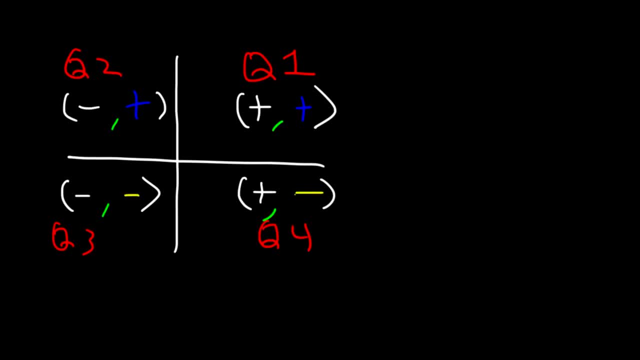 Sine is positive in quadrants 1 and 2.. Cosine is positive in quadrants 1 and 4.. Now you need to be familiar with the angles. On the X axis, the angle is 0 degrees. On the Y axis, the positive Y axis is 90.. 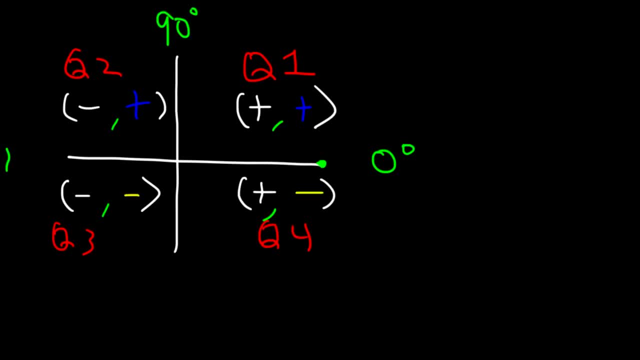 And on the negative X axis it's 180.. And on the negative Y axis it's 270.. If you're traveling in the counterclockwise direction, Now 0 and 360 are the same. They're coterminal angles. 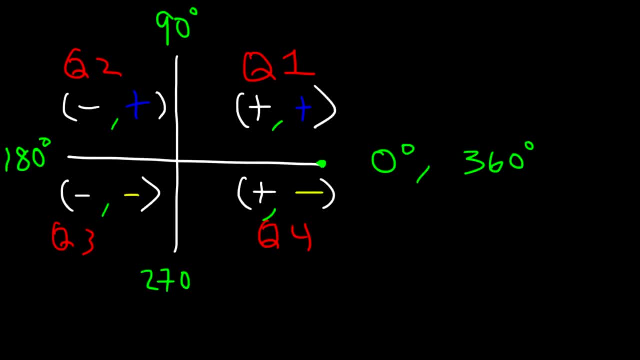 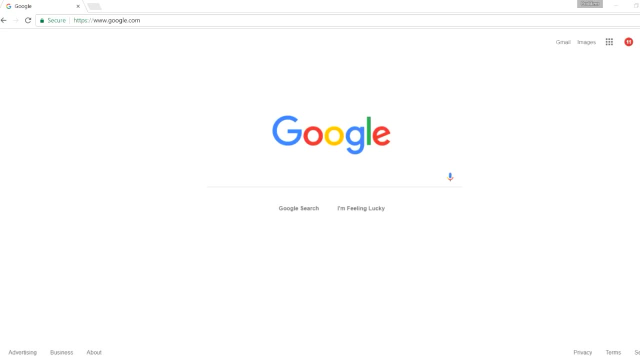 Which means that they land on the same position. They're different angles that point to the same point on the graph. Now, for those of you who want access to my complete online trigonometry course, Here's where you can find it: Go to udemycom. 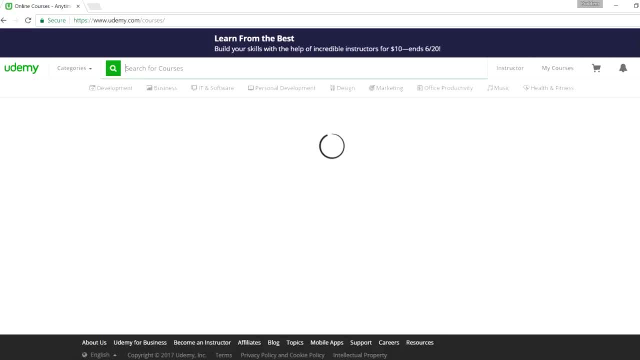 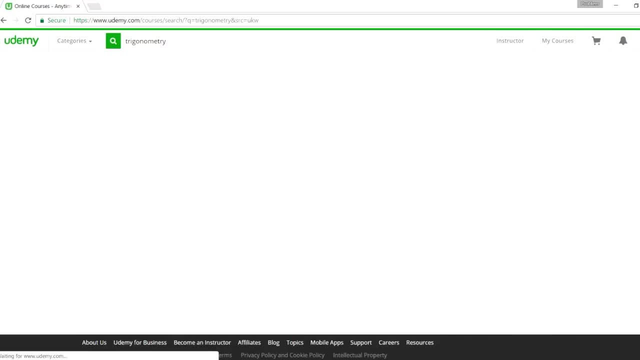 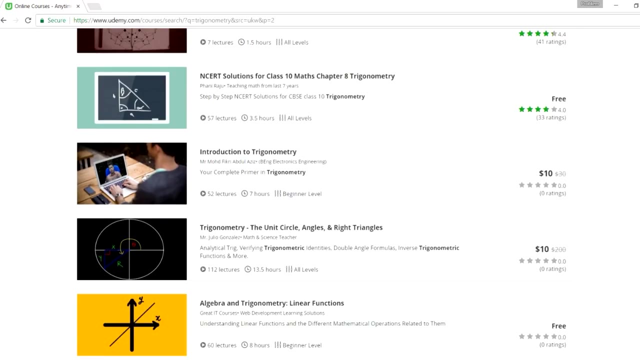 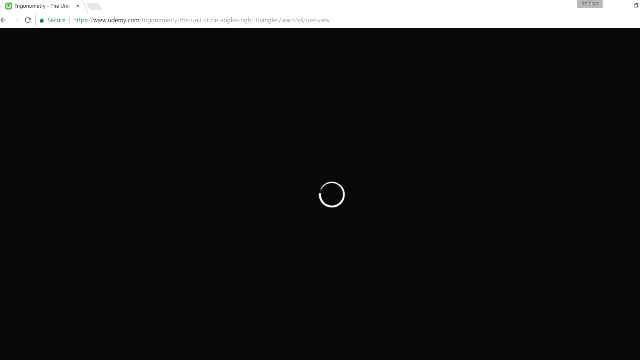 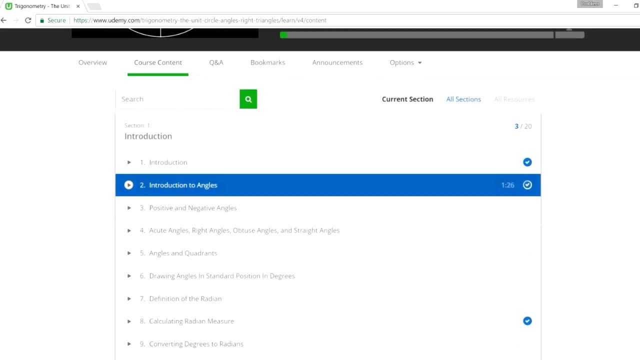 And then in the search box You can just search for trigonometry And you can see my course is basically the one with the black background, And then here is it. I'm still adding more lectures, But here's what I have so far. 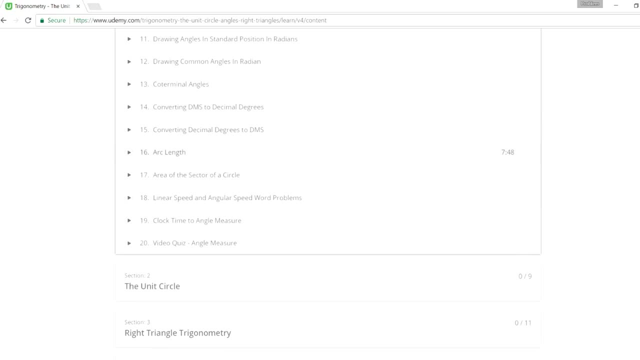 Introduction to angles: Drawn angles, Converting degrees into radians, Linear speed, angular speed problems, Arc length, Information on the unit circle. How to evaluate trigonometric functions Using the unit circle, Right triangle trigonometry- Things like SOHCAHTOA. 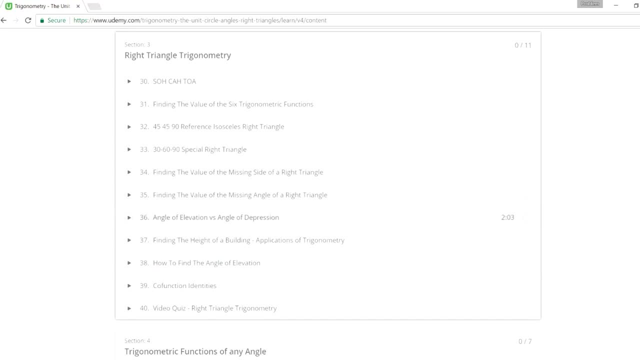 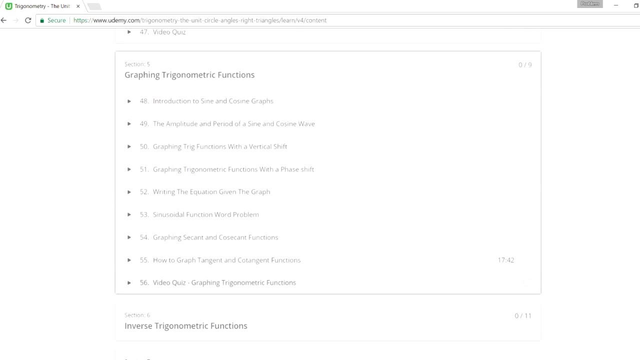 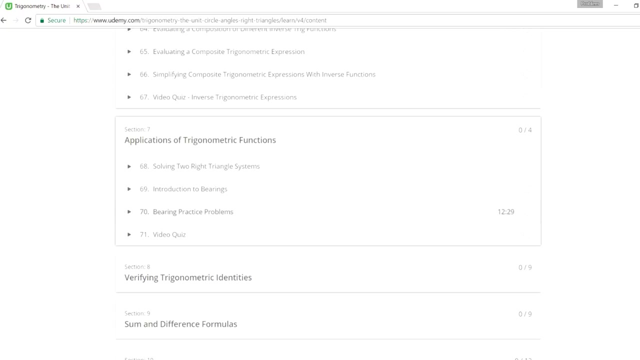 Even you can have video quizzes as well, Solving word problems Like angle of elevation problems. And then you have the next section: Graphing sine cosine functions, Secant tangent, Inverse trig functions- Pretty much all the common stuff that you'll see in a typical trigonometry course. 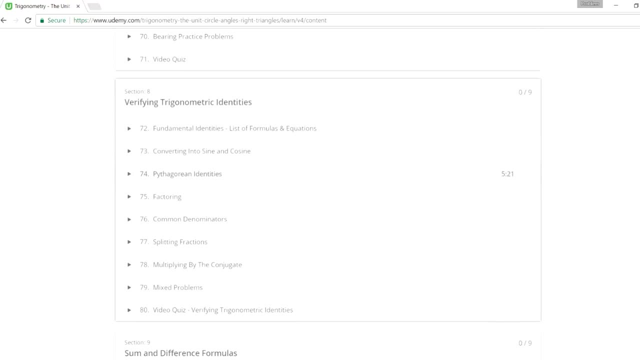 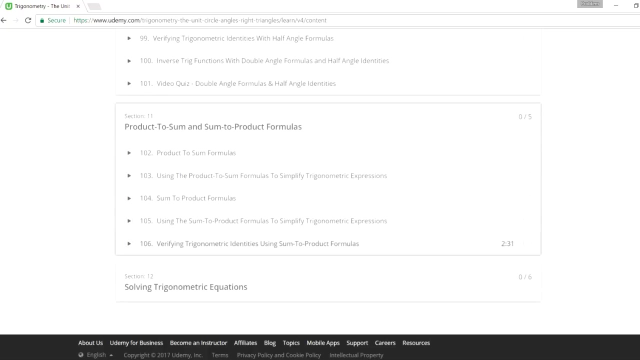 Even solving Behrens, Verifying trigonometric identities, Sum and difference formulas, Double angle, Half angle And some other things too, And, as I mentioned before, I'm going to add some other things as well, So feel free to check it out when you get a chance. 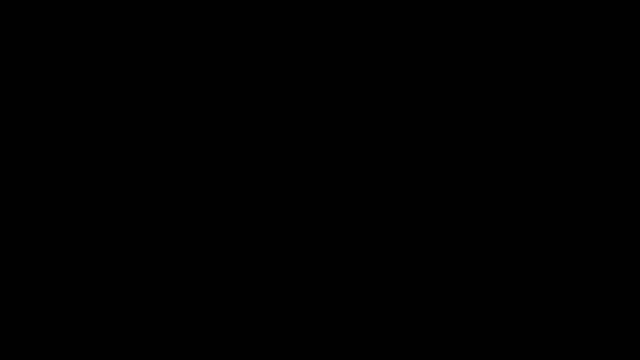 And let's continue back to the video. Now let's talk about how to draw angles in standard position. So how can we draw an angle of 45 degrees in standard position? So the first thing you want to do is draw your X and Y axis. 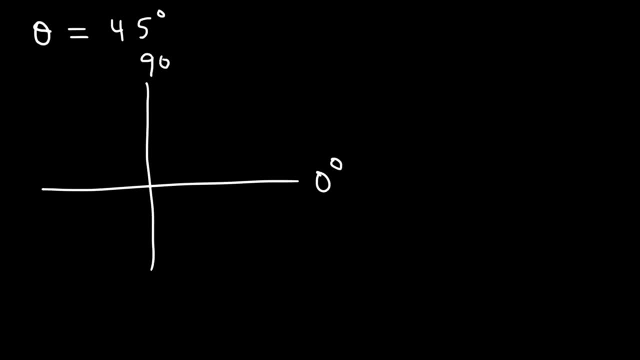 Now you know this is 0 degrees, The Y axis is 90.. 45 have to be right in the middle between 0 and 90. So this is the initial side Which I'll write- I for it- And the terminal side. 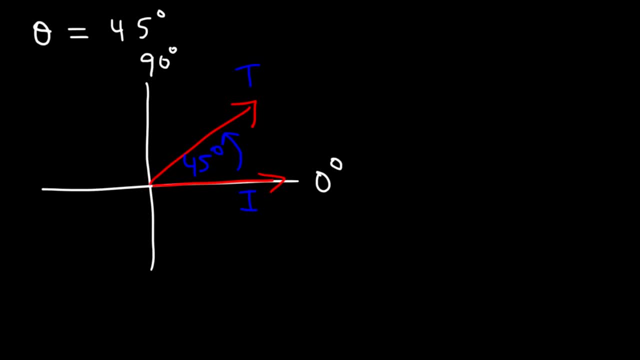 And so this measure is 45 degrees. Now for future examples. I won't always draw the initial side, But whenever you want to write the angle in standard position, It's always assumed that the initial side is on the X axis, So you might just see me draw the terminal side. 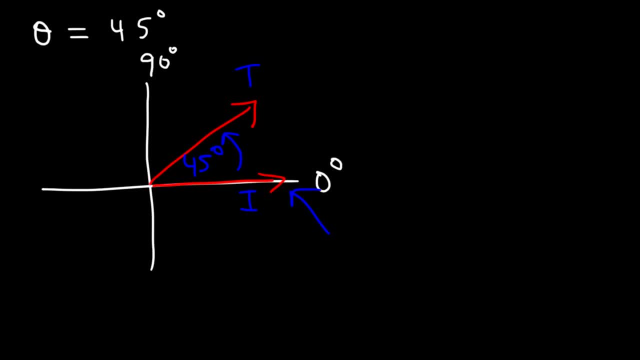 But keep in mind that the initial side is there, Even if I don't show it Now. let's try some other examples. I draw an angle of 30 degrees and 60. So feel free to pause the video and try it Now. we know that 45 is right in the middle between 0 and 90.. 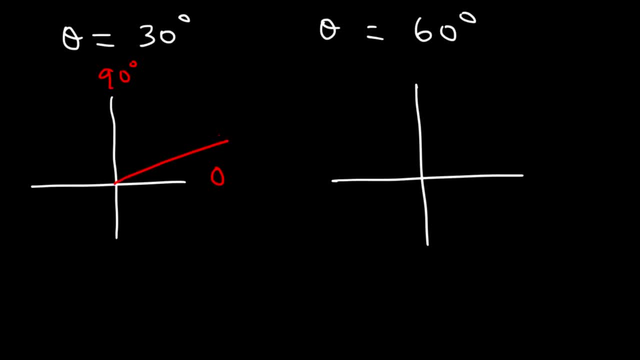 So 30 should be closer to 0 than it is to 90. So that should be an angle of 30 degrees. 60 is closer to 90 than it is to 90. So it should be somewhere in this region. So that's an angle of 60 degrees relative to the positive X axis. 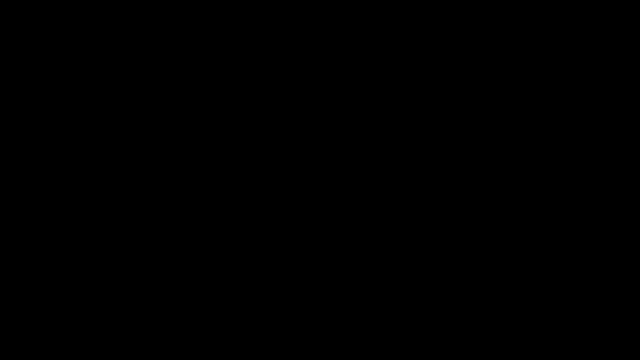 Where the initial side is. Now. let's try some more examples. Draw an angle of 135. And also 210.. And also try these: Draw an angle of 300. And an angle of, let's say, 330.. So feel free to pause the video and try these four examples. 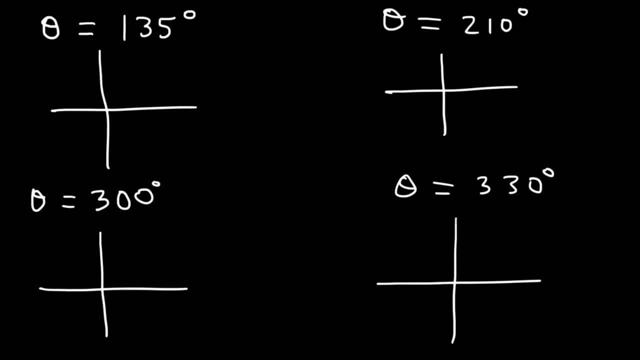 It doesn't have to be perfect, But as long as you have the angle in the right position and in the right quadrant, That's good enough. Now keep in mind: Between 0 and 90, the angle will be in quadrant 1.. 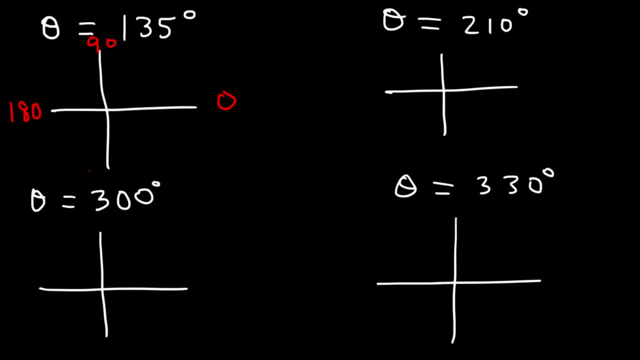 In quadrant 2 it's between 90 and 180.. In quadrant 3 that's between 180 and 270.. And quadrant 4 is between 270 and 360. Which is the same as 0. So 135 has to be between 90 and 180.. 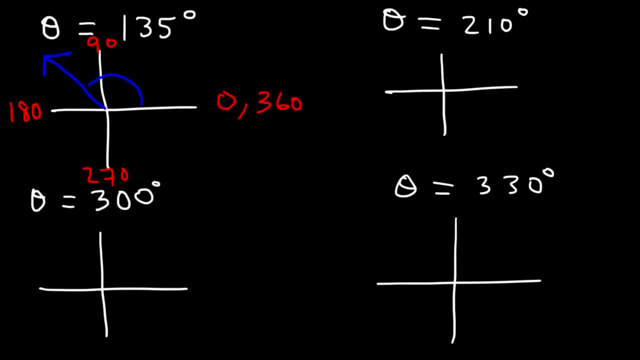 So it's in quadrant 2.. So this is an angle of 135.. Relative to the positive X axis. Now let's try 210.. 210 is between 180 and 270. But it's closer to 180. So therefore, 210 should be somewhere in that region. 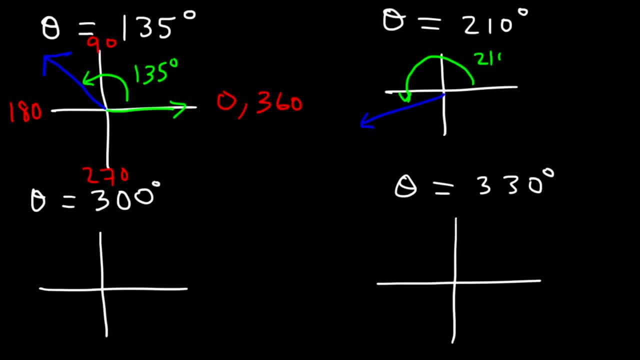 So this is an angle of 210 degrees From the positive X axis. Now what about 300?? 300 is between 270 and 360. But it's closer to 270.. The negative Y axis, So it should be in that vicinity. 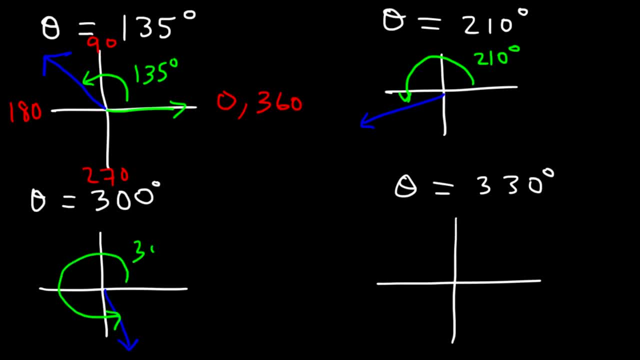 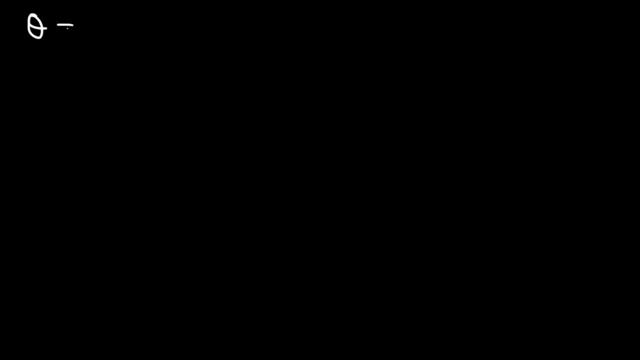 So this is the angle of 300 degrees, And then 330 is closer to 360. So this is going to be 330.. Now let's work on some negative angles in degrees. Go ahead and plot these numbers: Negative 60 degrees. 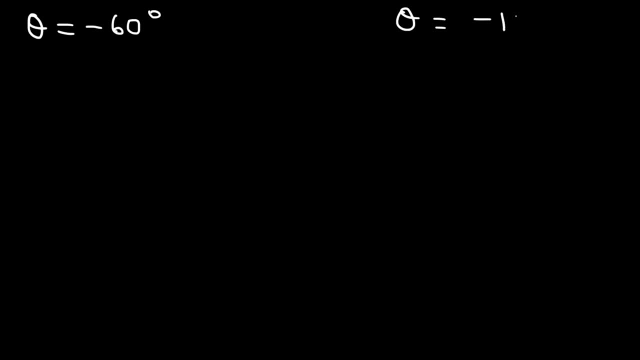 Let's say negative 135 degrees, Negative 180. And also negative 240. So go ahead and try those problems. So let's count the angles, This time rotating in a clockwise direction. So remember, This is clockwise rotation Actually. 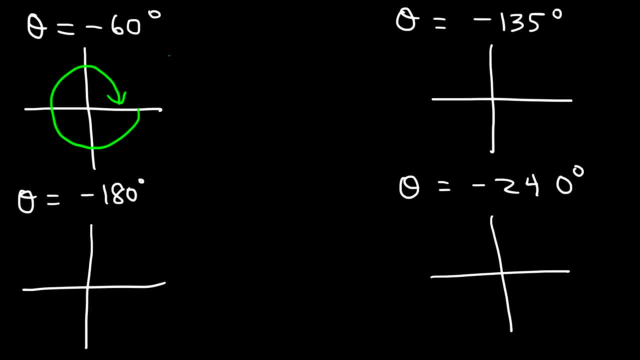 When you think of clockwise rotation, Think of the way a clock rotates. A clock travels in this direction. Counterclockwise is opposite to the direction of a clock. So this is counterclockwise. So just make sure you remember this. 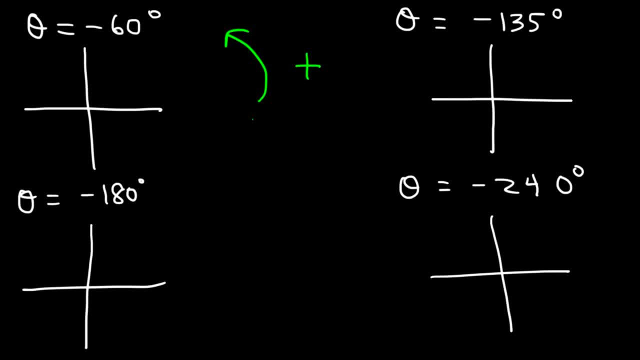 In a counterclockwise direction, The angle is positive. In a clockwise direction, The angle is negative. So we know this is 0. And this is positive 90. So therefore, This must be negative 90. Because we travel in the clockwise direction. 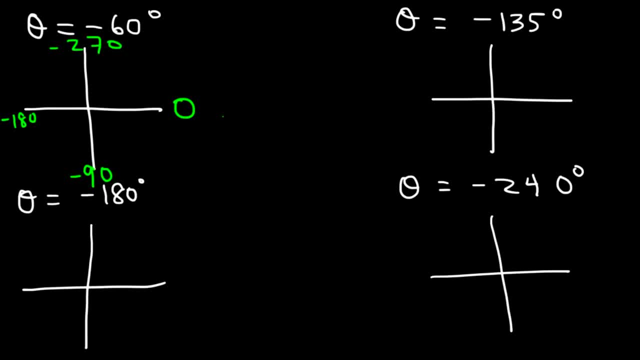 And this is negative 180.. Negative 270.. And 0 is equivalent to negative 360.. So we want to stop at negative 60. So we need to rotate close to negative 90. But not too far. So that's an angle of negative 60.. 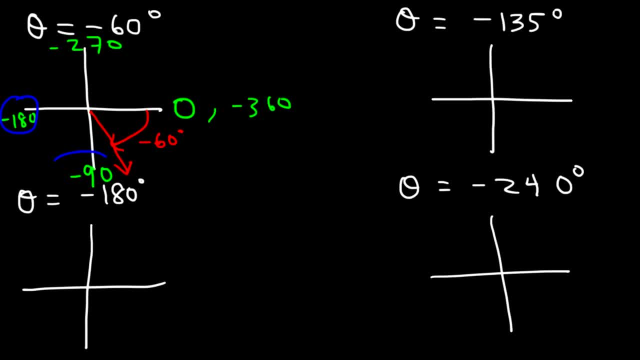 Now what about negative 135?? That's between negative 180 and negative 90. So negative 135.. It's in quadrant 3.. But it's right in between negative 90 and negative 180.. So that's negative 135..